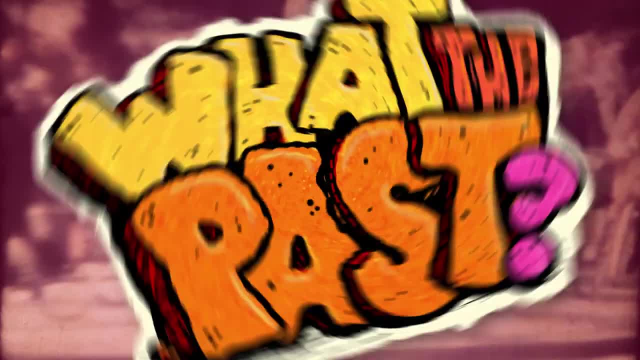 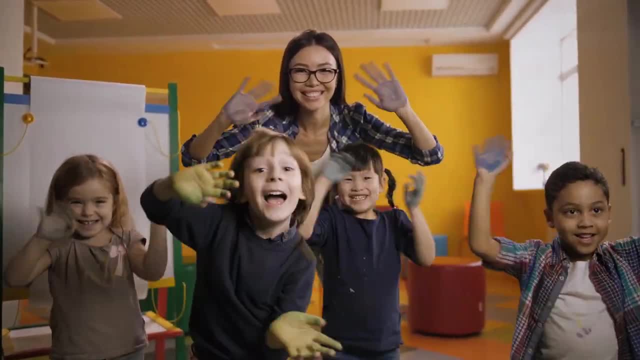 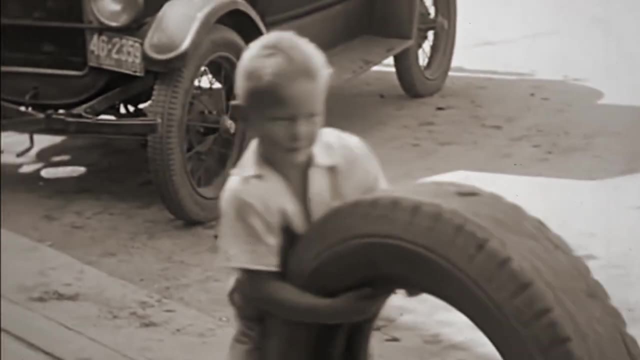 It's almost impossible for us to imagine what it might be like for kids not to have a childhood. But, believe it or not, for most of human history there was no such thing. Up until a few hundred years ago, being a kid tended to be brutal, Medicine was minimal and public health was. 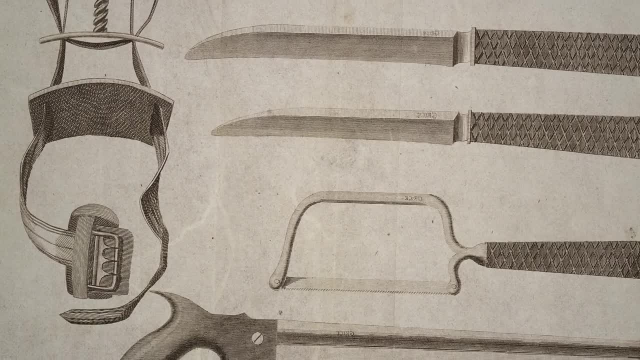 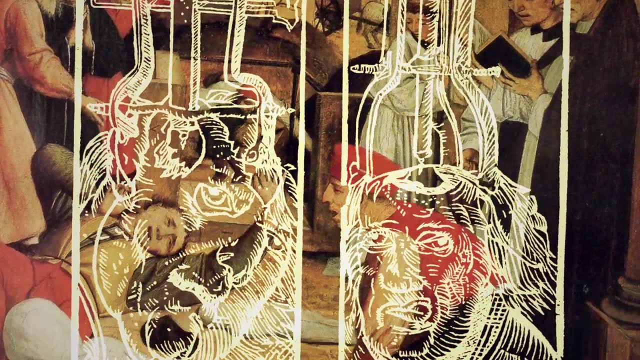 almost non-existent for most of Western history, which means lots of babies never made it out of infancy, And if they did, well, that's when things really started to get hard. You see, from the ancient world until around the 1600s, kids were basically considered to. 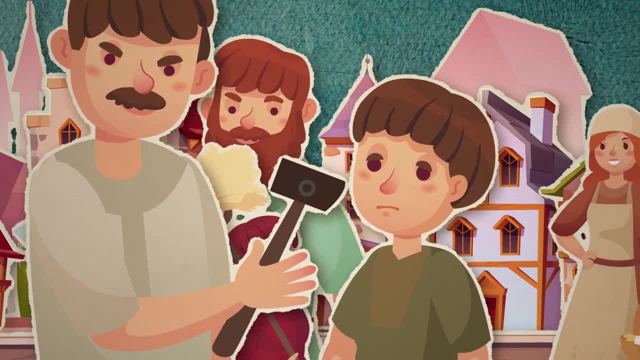 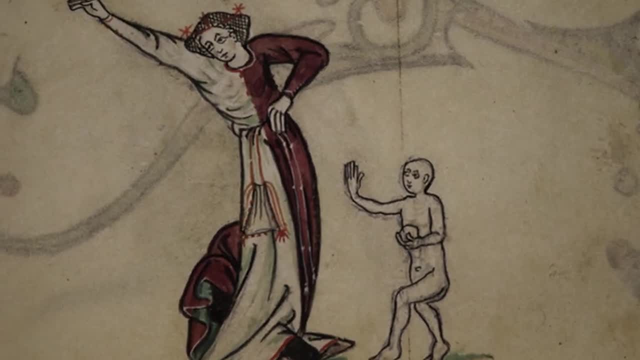 be small adults who needed to learn the ways of the world as fast as possible. In fact, you can see this in lots of medieval art, where kids tend to look like mini-adults rather than children. It wasn't so much that medieval parents were extra mean. 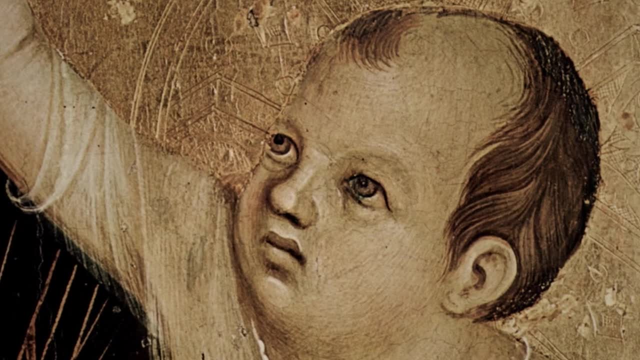 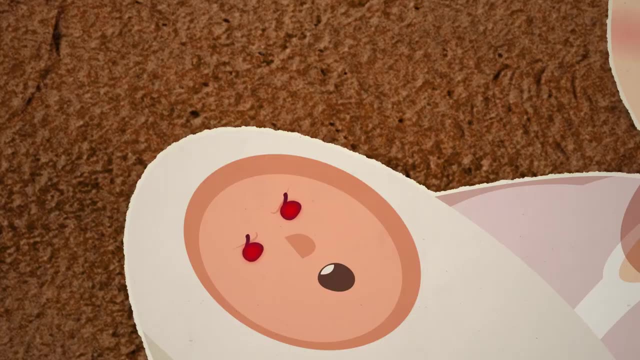 it's just that people at the time didn't really understand the concept of medieval art of being a kid, For instance. most people in the Western world at the time believed that newborns were actually evil Yikes. The idea was that a child was born sinful and 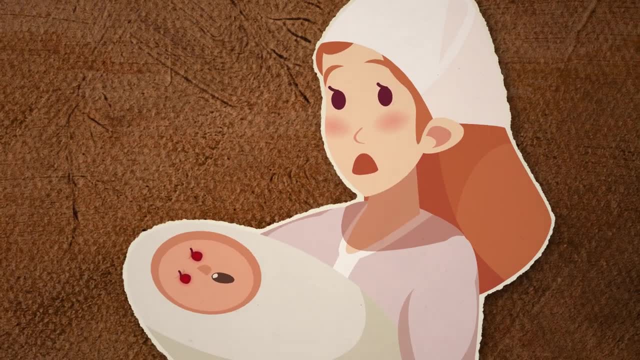 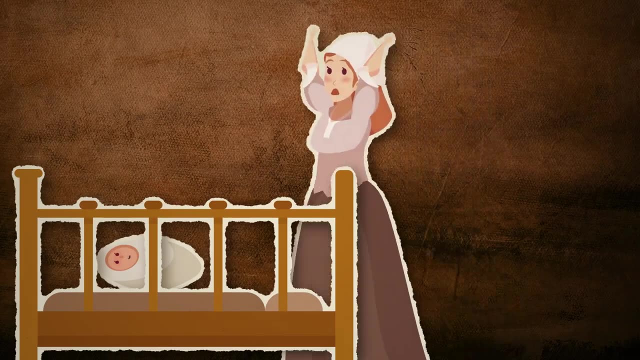 could only be purified through teaching. That's a lot to put on a baby, if you ask me, But that's what most people believed at the time, and the way they raised their kids reflected that, Instead of spending time playing with friends and scraping their knees, 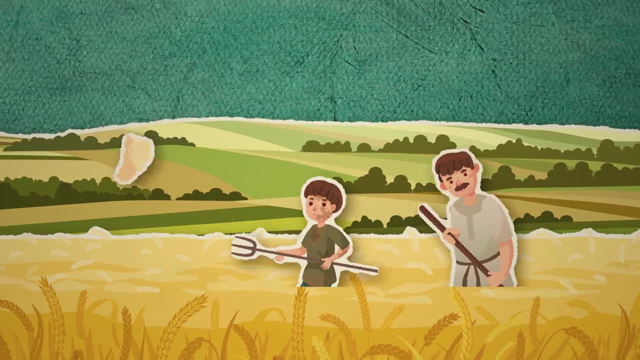 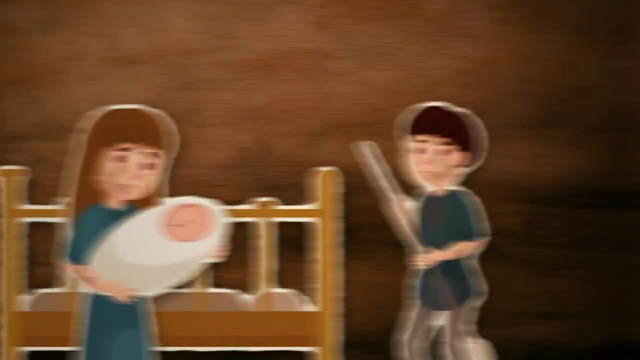 kids tended to scrape up the rest of their body working hard to help provide for the family, either working in the field or helping with tasks around the house, or most often, both Kids would start helping out the family around age five and would level up to more grown-up jobs as 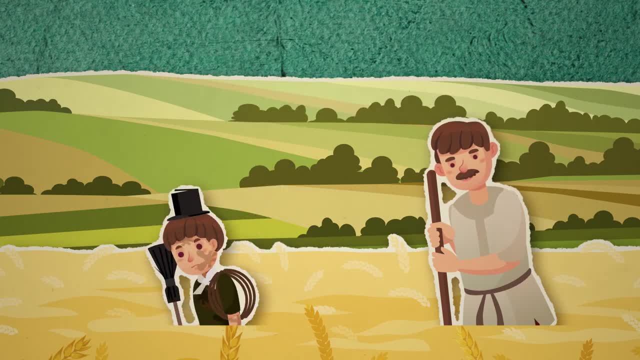 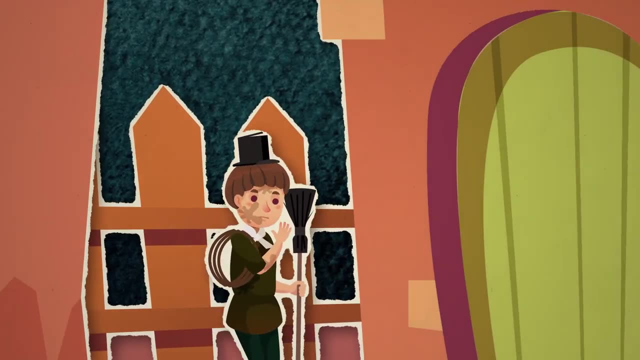 they were able. Most youngsters were also expected to go get jobs as soon as they could. A popular job for children as young as four in England was a chimney sweep. Since kids were so small, they had an easier time getting a job. But that wasn't always the case. Kids were also. 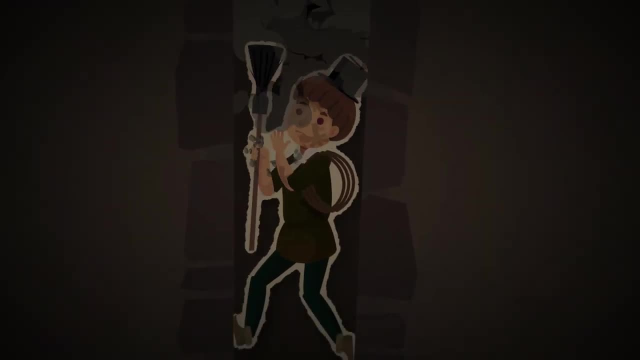 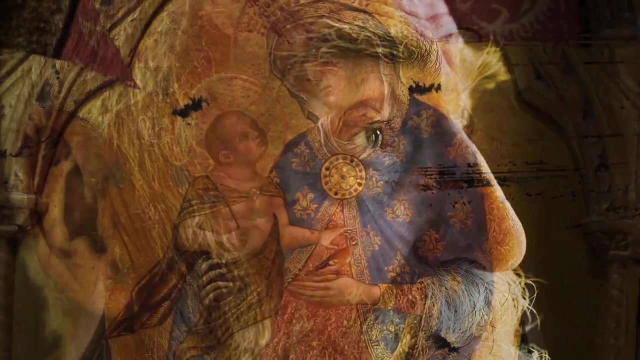 expected to go into the kitchen and sweep the chimney and in the meantime they had to do all the work that was left behind. The fact that this is incredibly hard and unhealthy work never seemed to occur to anyone, But thankfully for us all, that all started.